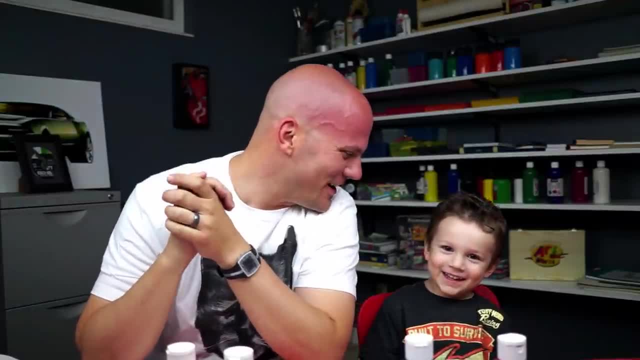 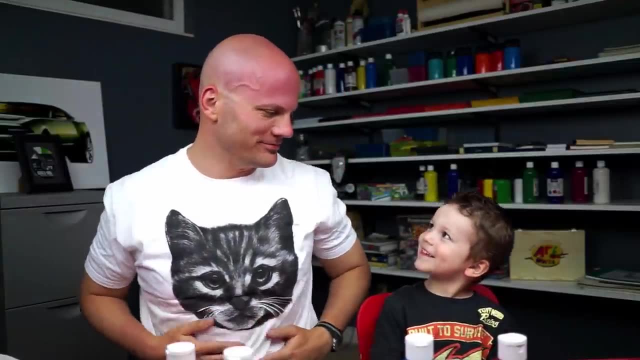 And sauce. We had ice cream Too. huh Yeah, Yeah, we had ice cream. It was a lot of fun. huh, Tastes good in our bellies. go like this. All right, we got paint. what kind of paint do we have? what color is this? 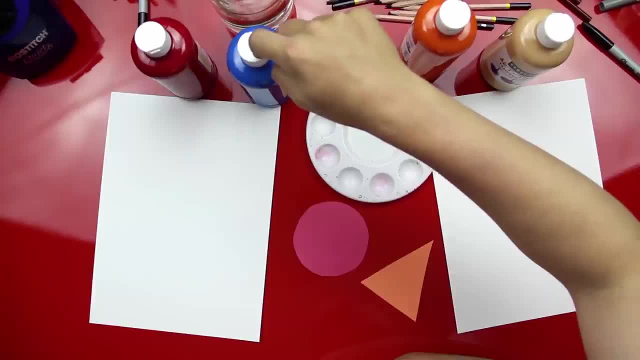 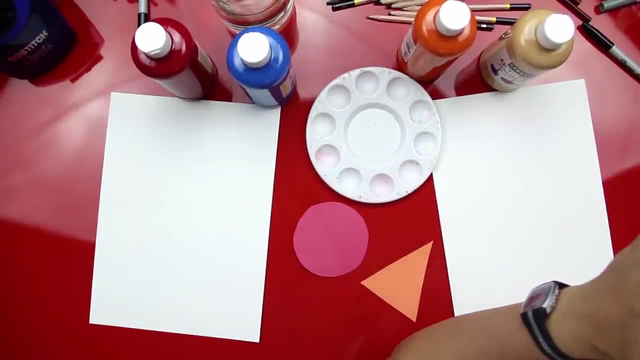 Brown. what's this one? orange, Blue and red. And we're gonna be doing special, We're gonna be doing some shapes, huh, Yeah, what's. what shape is this? Um, triangle, Yes, triangle. and what shape is this? Yeah, circle. and so this is a fun activity to work with your young artists on. 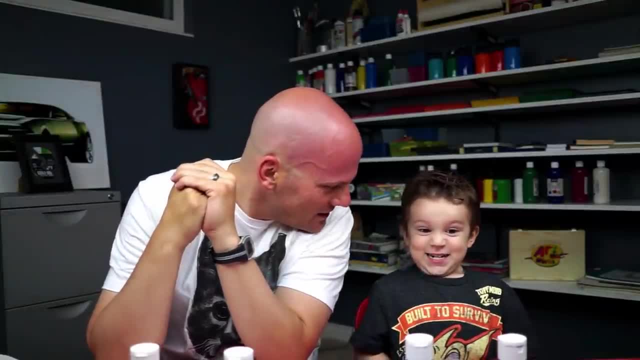 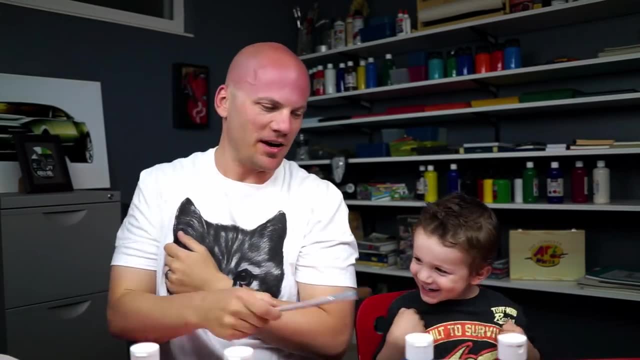 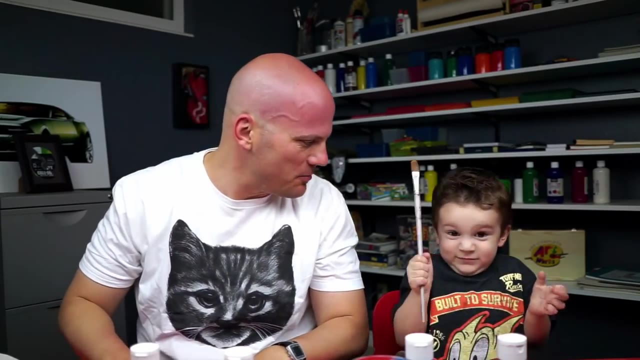 shapes and colors. Should we paint? Should we paint? Yeah, All right, going this, yeah, Yeah, Yeah, All right, Here's your paintbrush. All right, We also got some water and we got a paint tray and we got some special paint paper. 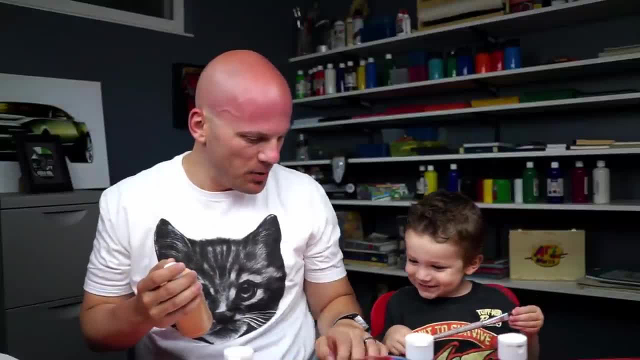 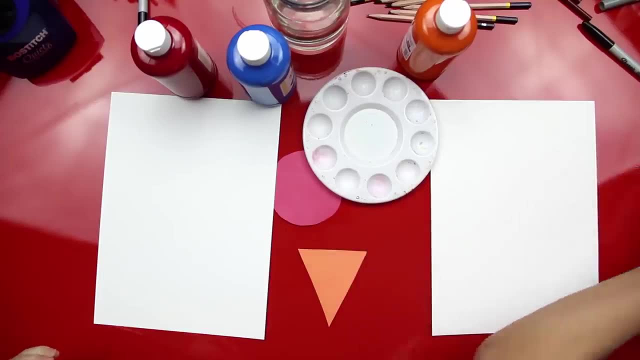 Okay, we're gonna paint a triangle. Yeah, we're gonna paint a triangle that looks like this, All right, and we're gonna use this color. I Think it's good with young artists to start off with not putting all the paint In your paint tray. Just start with the one you need first and then add as you go. 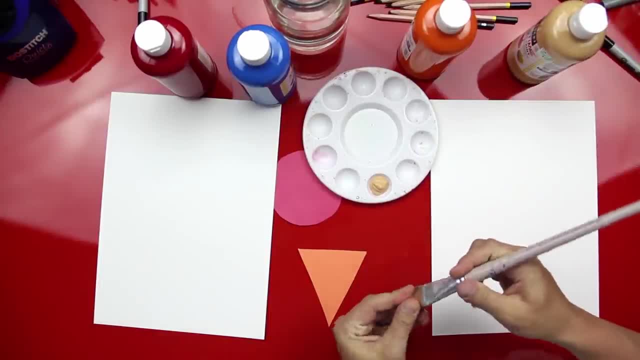 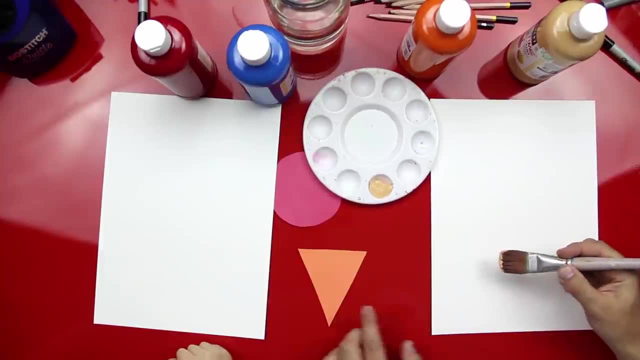 All right, watch me, Austin. Okay, watch me. we're, I'm gonna put a little. I'm gonna put a little water on mine. We'll get a little water on yours too. So watch this. Watch, I'm gonna paint a triangle. Paint a triangle like this, okay. 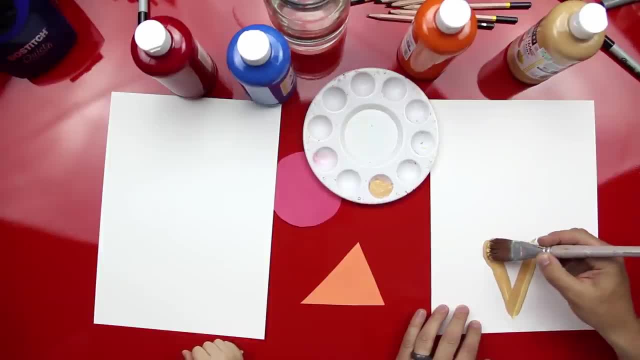 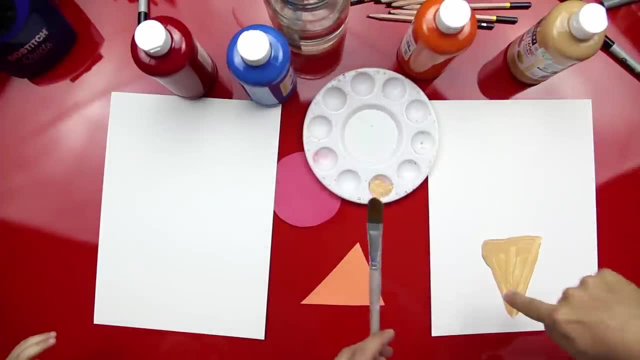 Okay, You go down and up and across and then paint it in. Okay, Can you do that? Yeah, This, what is that? What is this shape? What shape is that Triangle? A triangle, And it looks like a cone. huh. 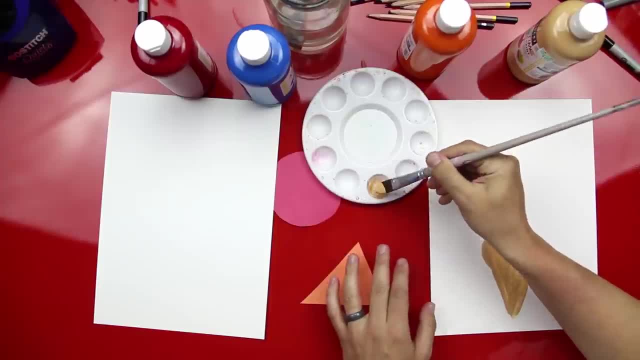 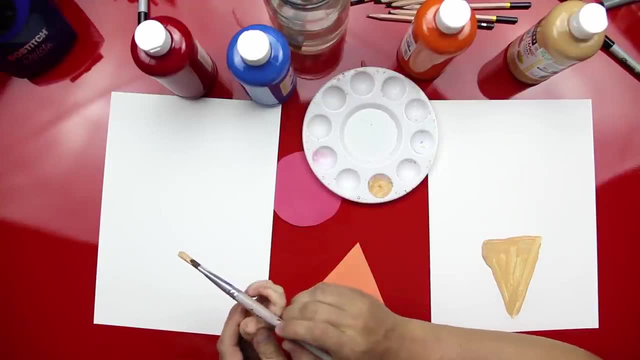 Yeah, Yeah, All right, Here you go, I'll let you do it Okay. Okay, Here's your paint. Okay Here, hold it like a pencil. Okay, Here, let go and hold it down here. Okay. 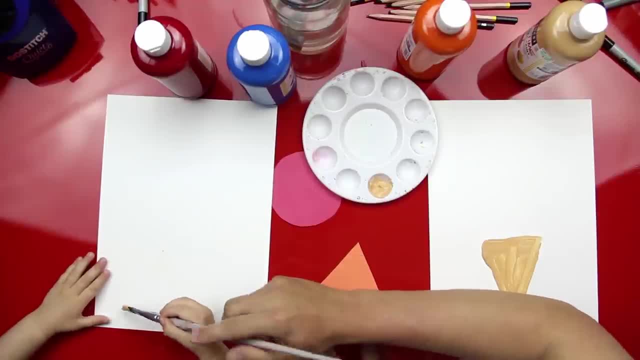 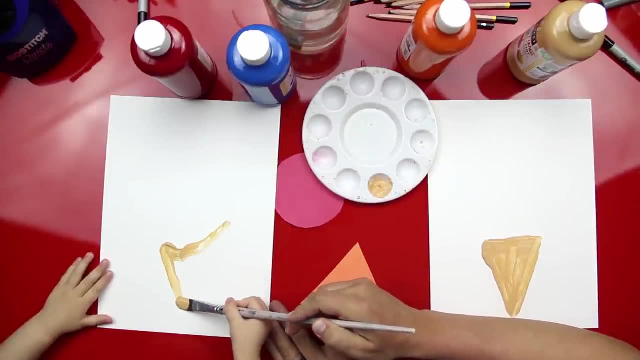 There you go, And so go down, down up. Okay, Start up here, Go down, Or you can go across. Let's go down down, And then we can flip it over and there's more paint, And then go back up. 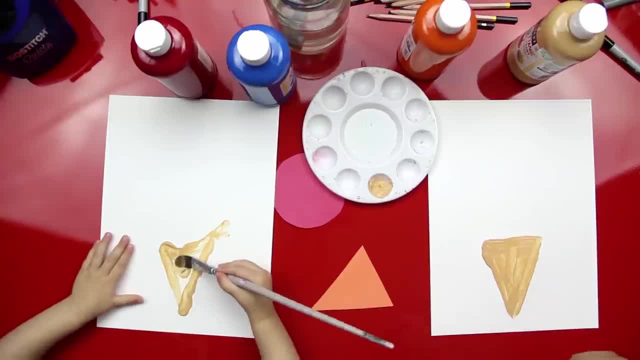 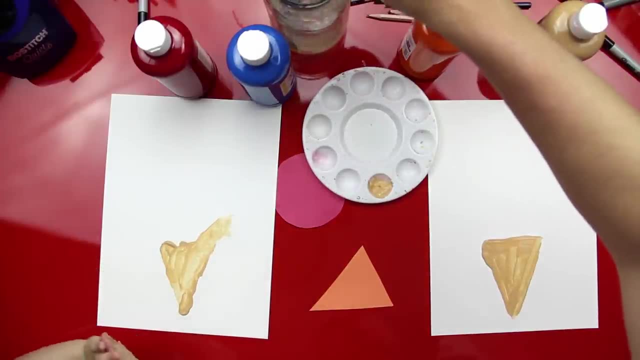 Okay, Can you color that triangle in? Yeah, Color, paint it in. There you go, Good job, Good job, Awesome Austin. Okay, Let's put some water in it and we'll get some more paint. What color should we do first? 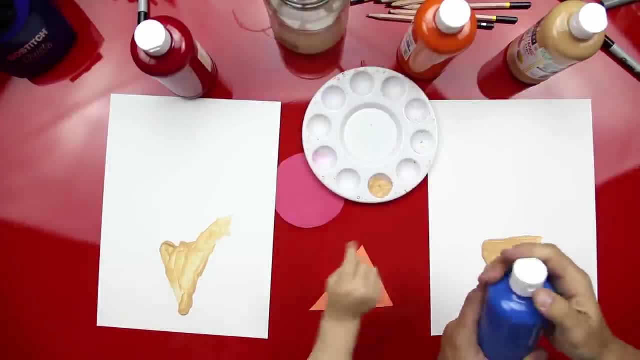 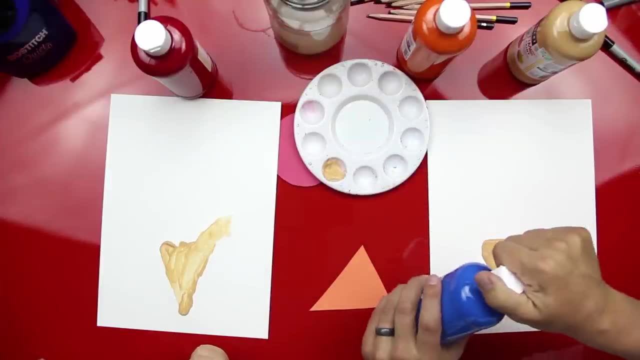 Blue. Yeah, All right, Let's do blue And that one, And I'll put it in that one. And what shape? We're going to do a different shape now. huh, Okay, We're going to do a different shape. 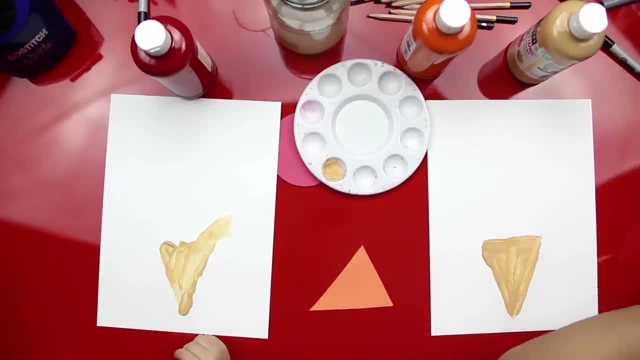 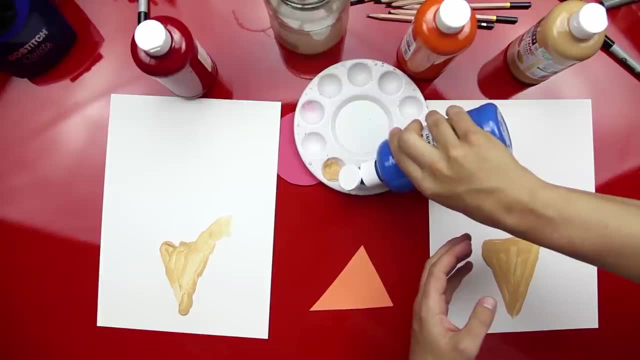 Yeah, Okay, What shape should we do? Um, this circle? A circle? Yeah, Let's do a circle. All right, Here's the blue. Okay, Get some blue on there And watch that, Okay, Okay, I'm going to rinse it out. 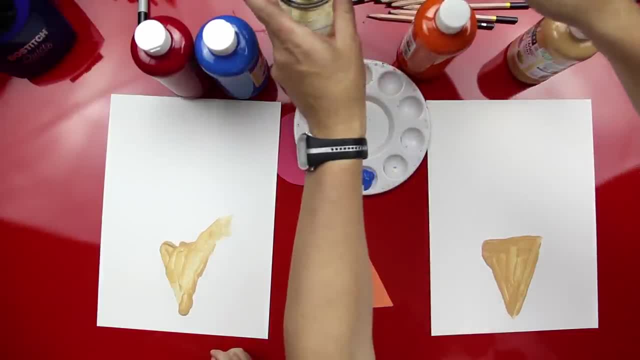 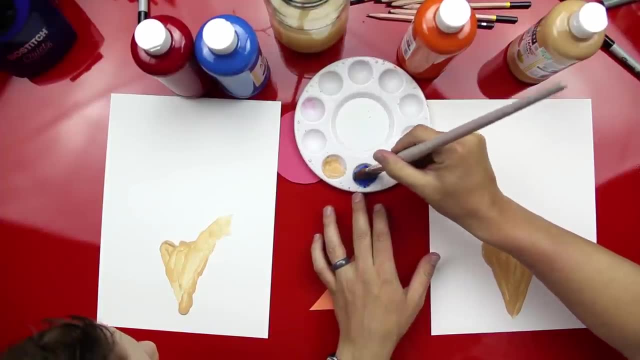 I'll get your paintbrush in just a sec. Okay, And you're so excited, huh? Yeah, All right, We'll dry it off. Okay, Watch this. I'm going to do a circle, all right, Okay, You ready. 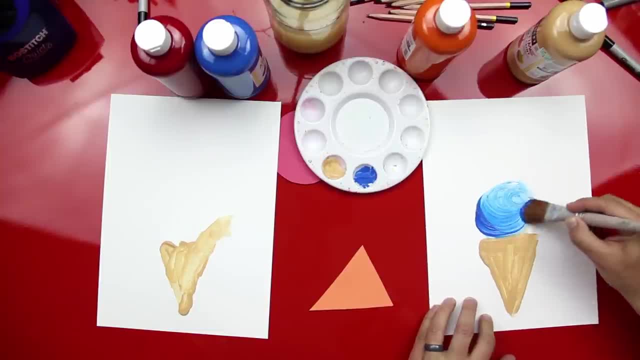 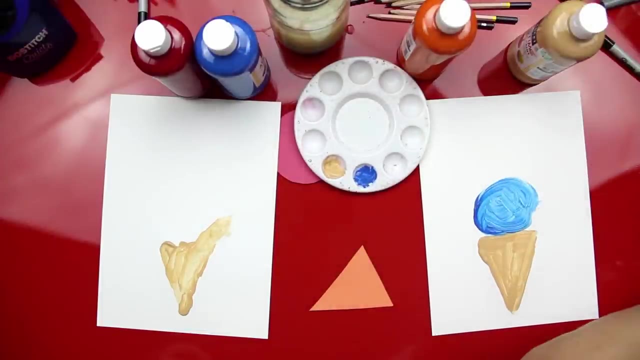 Yeah, Do a big circle. I'm going to do a little more paint. Does that look like a circle? Yeah, Yeah, All right, Let's get your paintbrush. I'll get it here in just a sec. Dry it off a little. 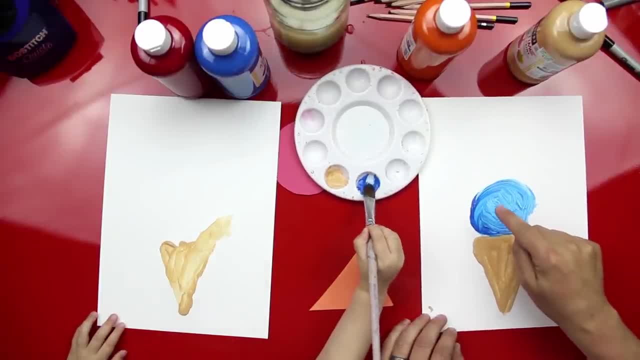 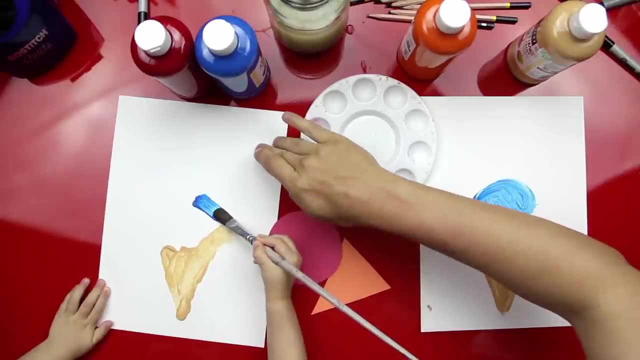 All right, Get some blue, Okay, And then we're going to do a circle like this: Okay. Okay, Start up here on the cone and do a circle. You do a circle. Yes, I'll help you a little bit. 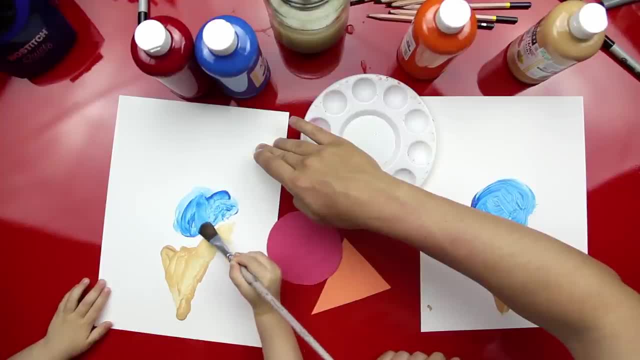 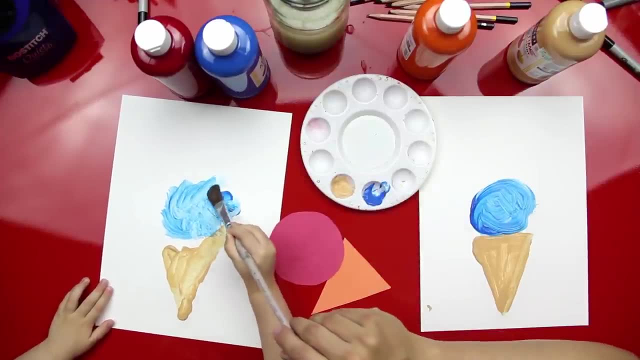 There you go, Color it in, You do a circle. Good job, Awesome, That's awesome. All right, Let's put it back in the water. All right, Maybe we'll just do. Let's do one other circle on top. 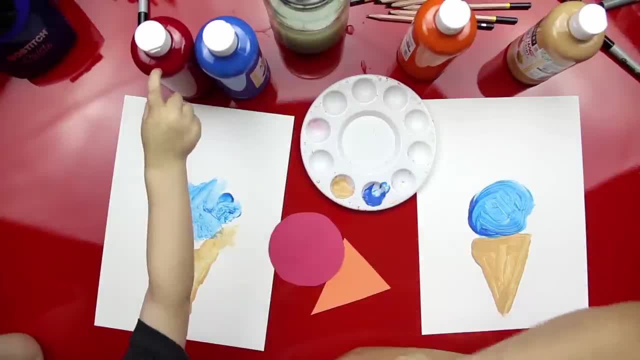 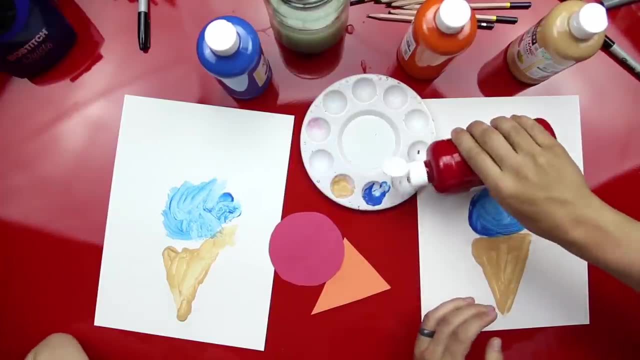 We were thinking we'd do two, but let's just do, or I mean three, Let's do two. Should we do red? Yeah, Okay, Okay, I will. Here we go A little red. You want to watch dad do it? 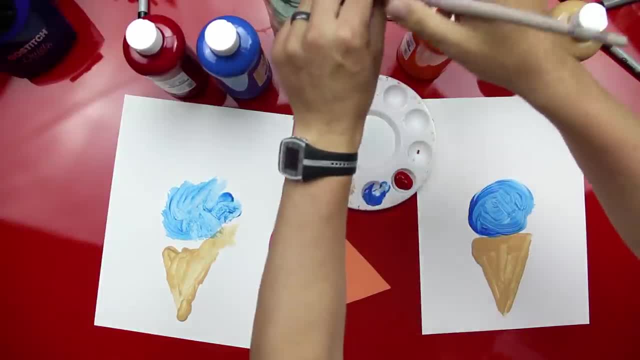 Yeah, All right, That'll do it first and then you do it after me. Okay, All right, Here we go, Get a little of that water off and get some red, Okay, And then we'll do this one, All right.